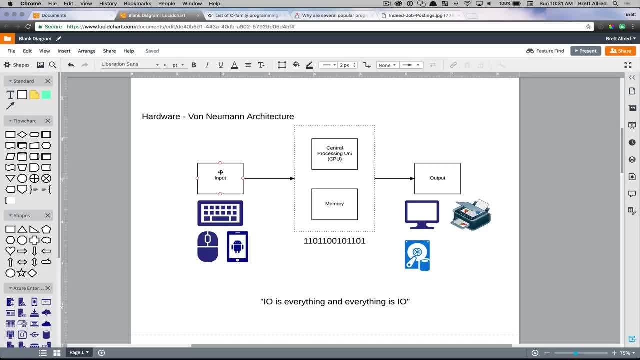 move it around. it gives input to the computer where to move the cursor, whether to go up or to go left or to go right. that's giving input to the computer. A more modern example of input would be a smartphone that has a touch display You can type in, using like a digital keyboard, into the computer or 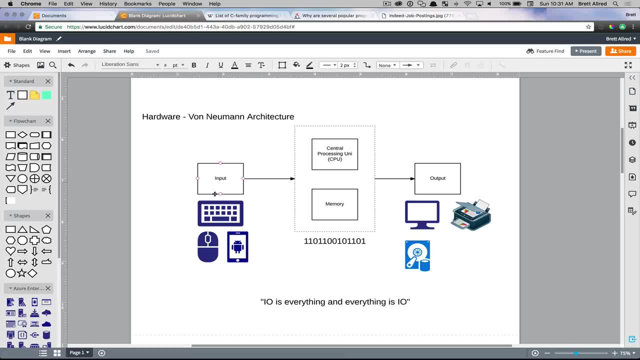 you can use gestures with your finger, but that's all with the phone and the touch gestures that are used. So there's other input devices, but the most important thing is to remember that there's a big category of hardware that we consider input devices. That input then goes into the computer, which the computer consists. 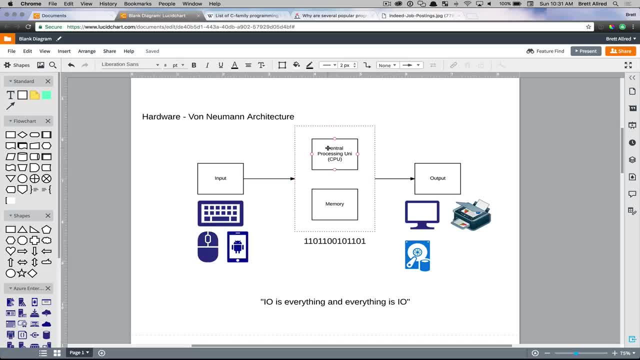 of two major components. One is the central processing unit. You can think of that as the brains of the computer. that does all of the calculations. It's doing the addition and the multiplication and it's moving things around in memory. It's really orchestrating everything that. 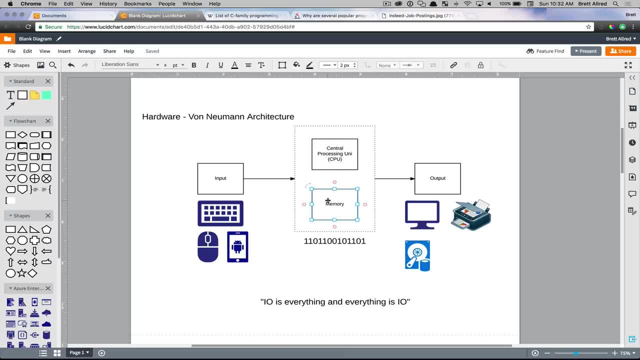 happens in the computer. And then there's memory and that's just internal storage in the computer so it can remember what it's doing, And we'll get into that a little bit more in future lessons. but memory is just storage that exists in the computer for the, the central processing unit or the CPU, to 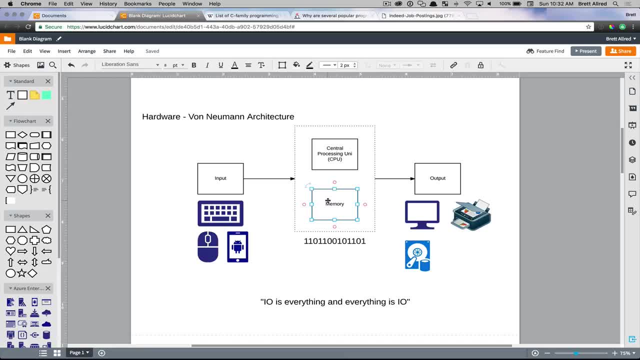 work with. Then, once it's done doing its computation and its calculation, it needs to take that data and send it to an output So it could output it to a computer. It could output it to a monitor, Put it to your screen, You could send it to a printer or you. 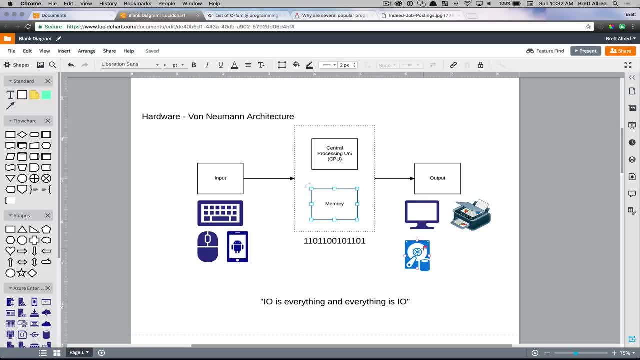 could send it to a hard disk drive to save for more long-term storage. And so this system of inputs, computation and outputs is really the basic, the basis of all computers and computer science and how it works. And so there was a mentor that I had that he told me this little phrase that is I owe is everything, and 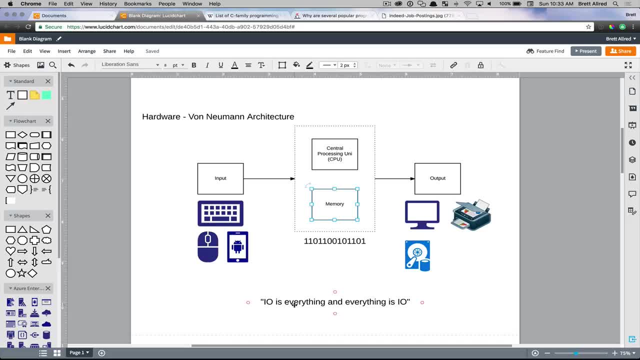 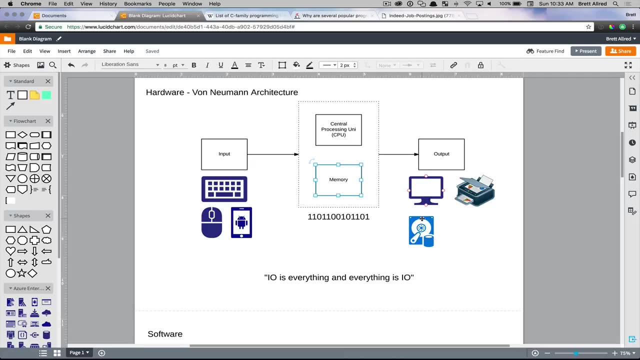 everything is I owe, And I owe stands for inputs and outputs, And really in computers, I owe is everything, and everything that we're doing is either an input- some type of computation- or an output. So let me give you an example here. If I open up a text editor like Atom, I have an input device which is my. 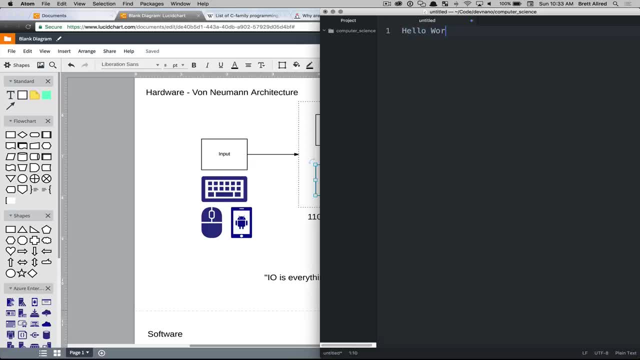 keyboard that I type in hello world, That's going into the computer, It's getting converted into ones and zeros and then it's getting outputted to this screen. And so that's an example of input going into the computer for processing and then output to a screen. Now, if I was to click file and print, I could print. 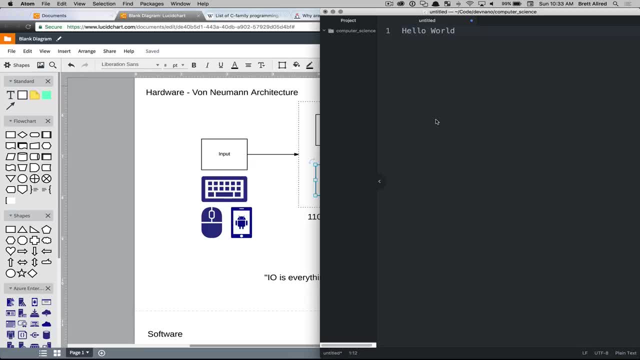 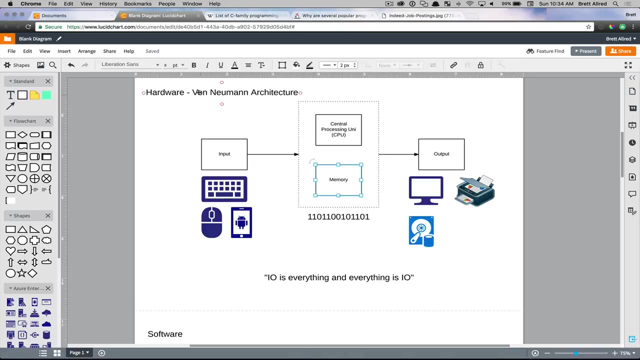 this to a printer and that would be going to an output device. Or maybe I could save this and email it to somebody and it would go out of my computer through a network card onto the internet And it would go out to them. So study a little bit more on your own time with the von Neumann. 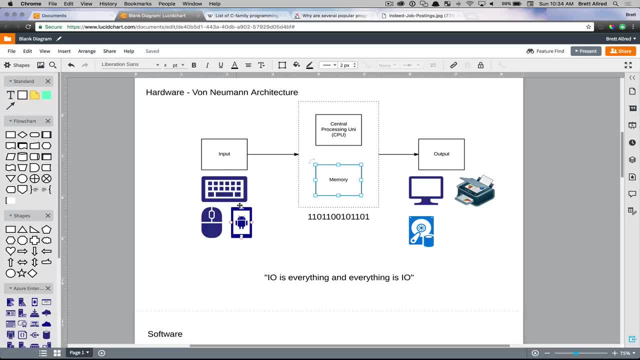 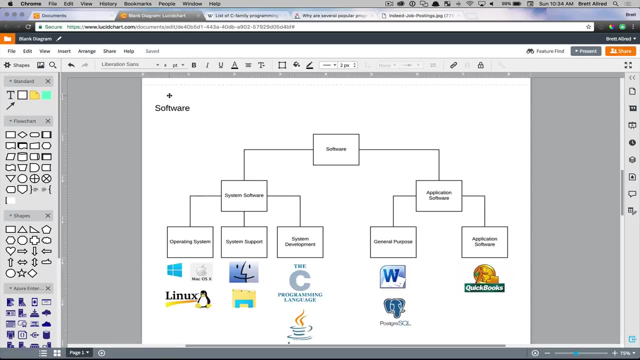 architecture. You can learn about this idea a little bit more of inputs, computation and outputs, But really this is everything that we're having to work with, And that's a good example of what's happening with the hardware. Now software gets a little bit more interesting. There's lots of kinds of software, So I 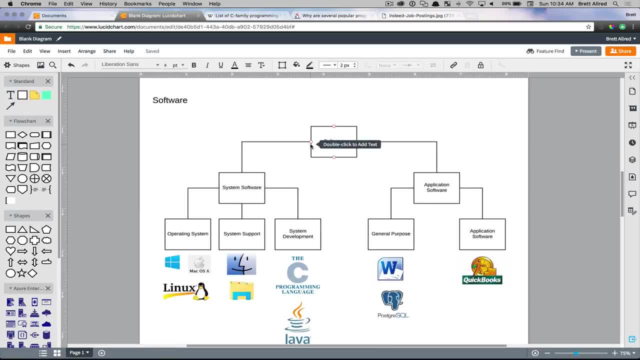 built this little tree to represent different types of software that exist. So off this left branch we see software, So I'm going to go ahead and go ahead and go. add that to the list. We see system software, and the most basic piece of software is the operating system. So you're probably familiar with Windows as 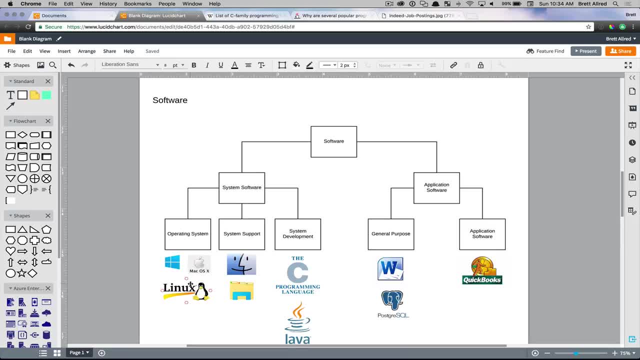 an operating system, or maybe Mac OS X or potentially Linux, as the three major operating systems that exist. Now there's other operating systems, but those are the main three. Next, there's system support software. So if you're on a Mac, you can think of finder, which you can open up and browse the files, and it helps. 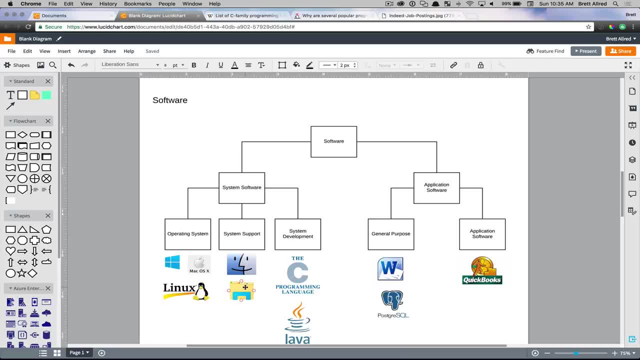 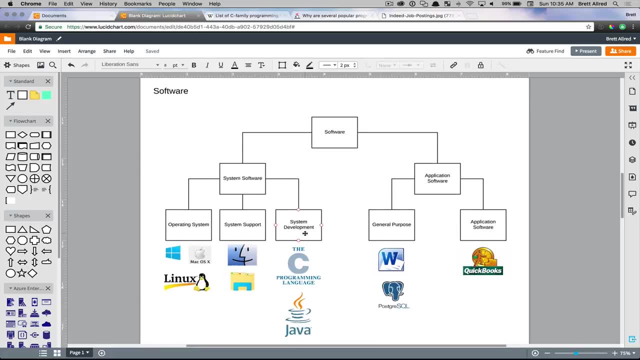 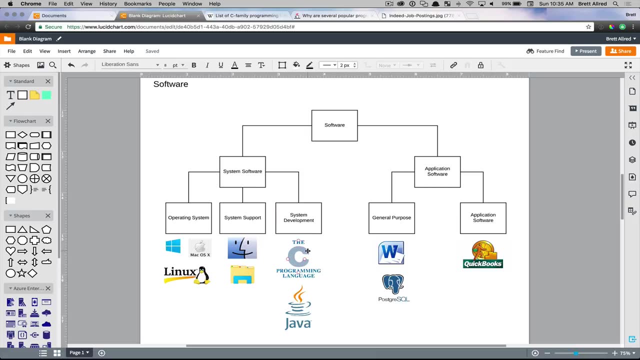 your system. in Windows there's Windows Explorer which will help you do the same thing, but just on Windows. then we have system development software, which actually allows us to develop software for the system. so you can think of like the C programming language with you have the language and you have the compiler. 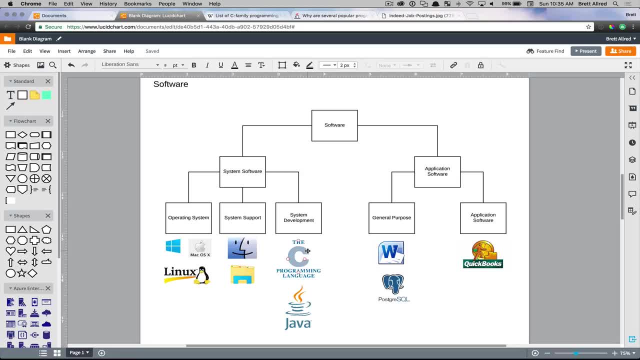 and you have the linker and the loader, everything that goes in to help you create software. Java is another example of system development software. they have different programming languages. you have the Java programming language and then the Java virtual machine. all of this and a bunch of different tooling to help you. 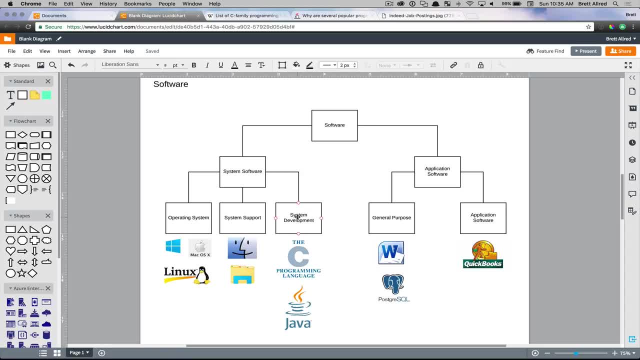 develop system software or to develop software in general. moving off the right branch, we have application software, which you can really break those into two sections, maybe more, but for our purpose there's general purpose software, which is software that does a lot of different things. it's, it's used for a general 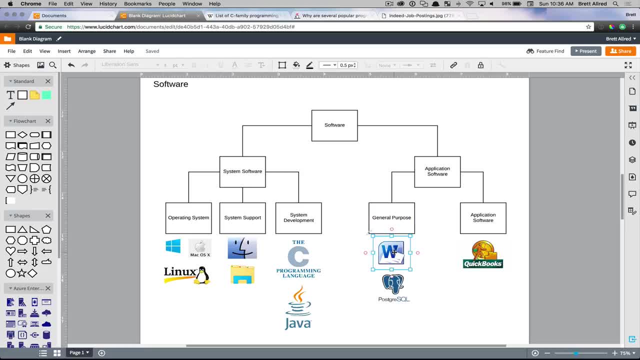 purpose. so Microsoft Word might be an example. on Mac, I think they call it keynote. well, they have keynote numbers and pages. pages is the equivalent to word, where you can use it for a lot of different things. you could write a book in it, you could create a presentation in it. it's really just. it can be used for. 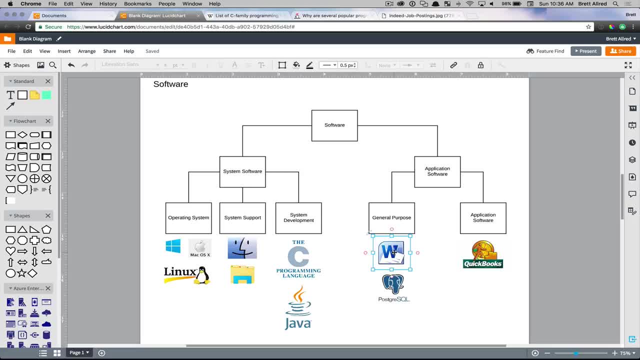 any function you could. it's almost limitless what you could do. another example is a database. database is general purpose, because there's lots of different ways that you can use a database for whatever your need is. then you have application software. this is more specific to a function, so I think of QuickBooks as an example. if you don't know what QuickBooks 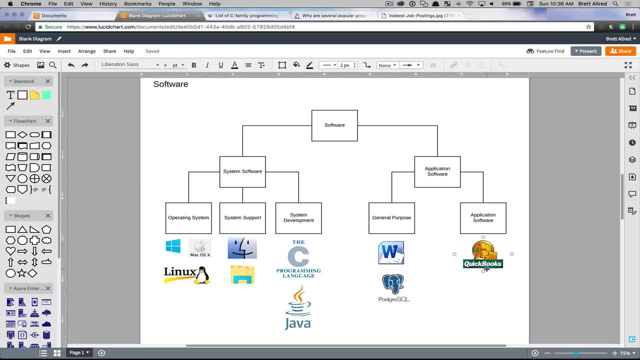 is. it's used for accounting and so it's very specific for accountants to go in, manage their ledger, manage their books, figure out all of the do the different reports for accounting, but it's very focused on accounting, so that's. that's specific, a specific application. so when we're writing, 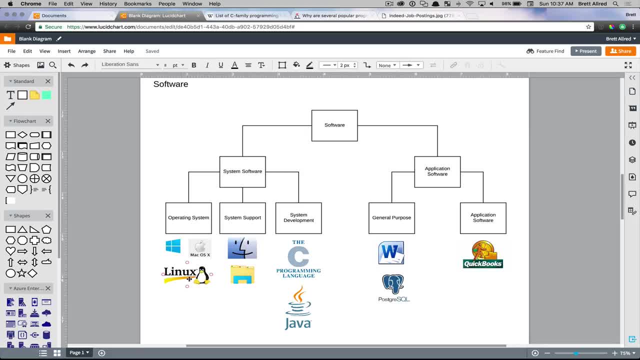 software. it's interesting to think of these things because you have an operating system to work with. you have system support software, you have system development software, there's general purpose software, application software, all of these things that give you ideas on what you can do for your application. 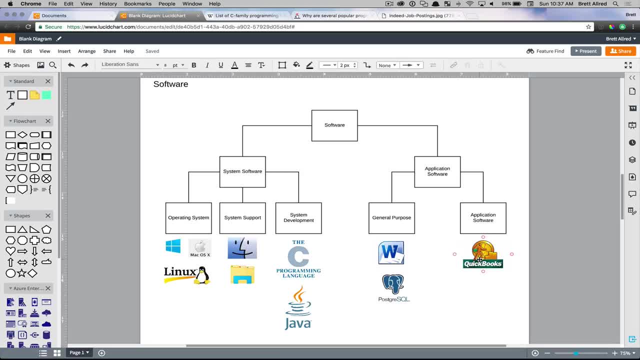 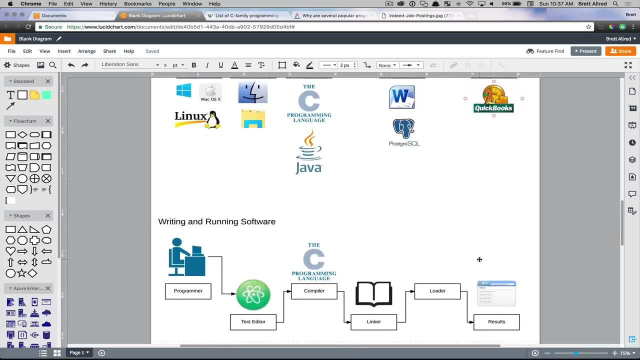 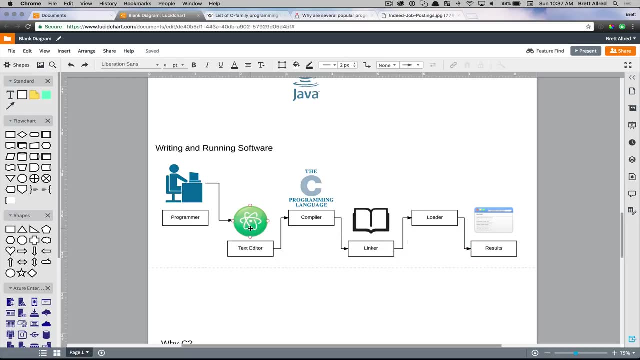 and you can leverage what's already been created to help you build up your application. so one last concept before we get into writing our own software. I want to talk a little bit about the process of writing software. so we have a programmer that gets a text editor, and in some of the previous lessons we've 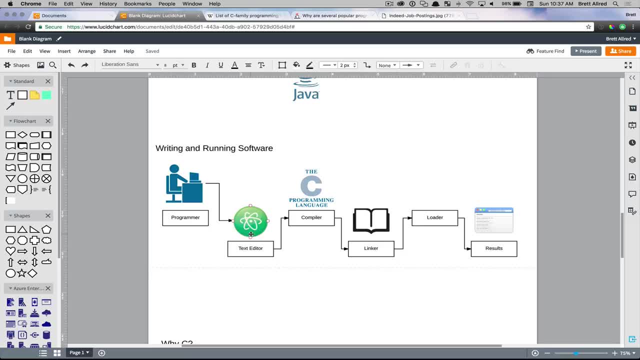 been using the atom text editor and he'll type in all of the different codes into the text editor and then he'll use a compiler to take that and we're going to use the C programming code and we're going to use the C programming code and. 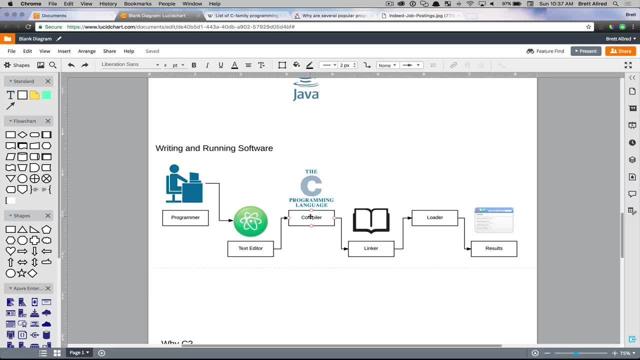 we're going to use the C programming language with this C compiler and he'll convert that down into the machine code. now, before that happens, there's a linker process which takes any other library software, like software that is going to use to help you out- and it will. it will link that and bring it in to your 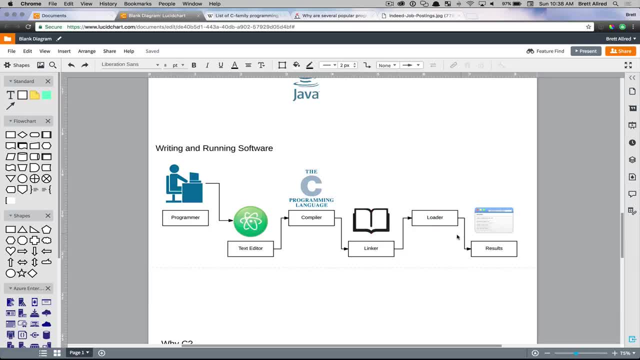 program, then it goes into this loader, it runs it and then you see the result. so we're going to go through this process over and over and over again, where we're typing code, we're compiling it and linking it, this will and loading it. this will happen in basically like one phase, and then running it will be the third. 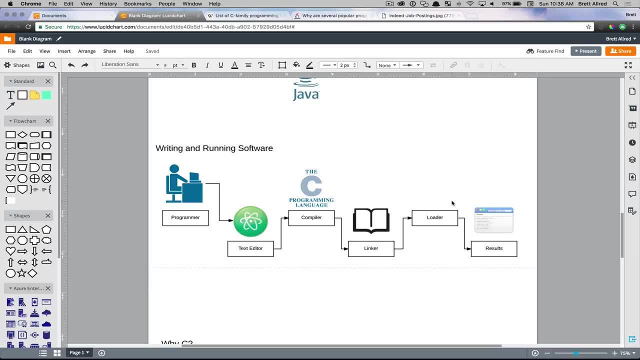 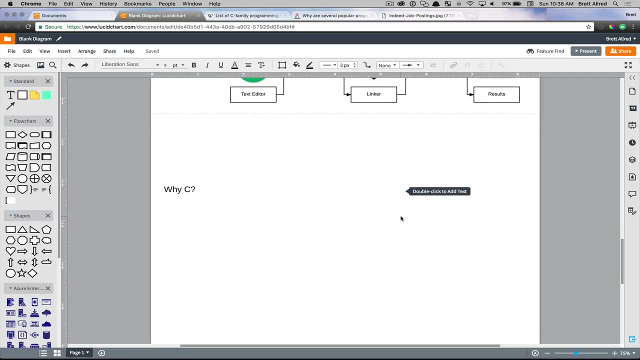 phase and you'll see how we program, we compile, we run, we program, we compile, we run, and that's, that's the process of programming. now, to teach you, we're going to use the C programming language and people ask me oftentimes why C? and I like to teach C or use that as the basis of computer science and learning. 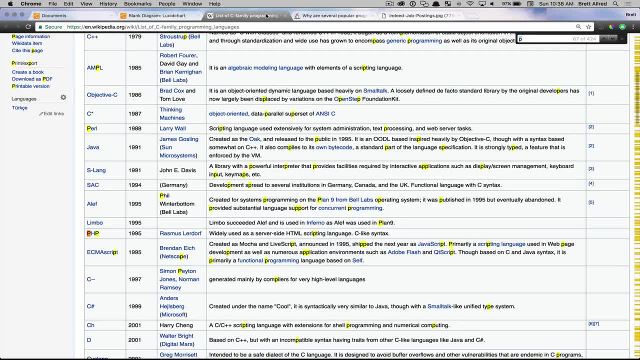 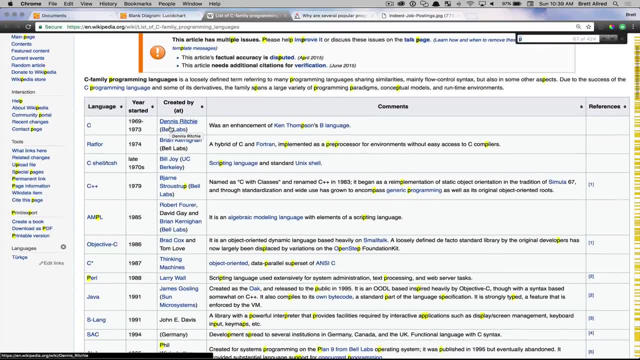 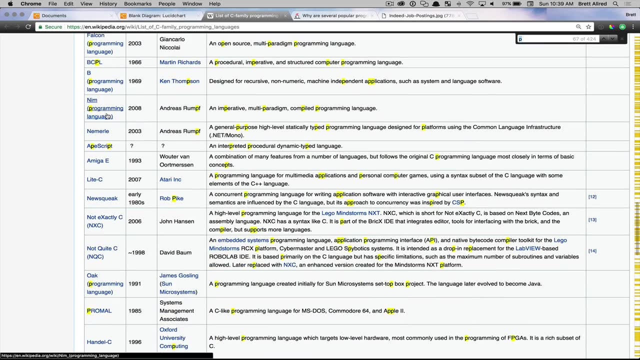 programming, because if you jump over to Wikipedia you're going to see a whole bunch of different programming languages that are based on C. so if you jump through here, all of these new programming languages have their roots or their basis in how C has done things. you go through here and there's- there's. 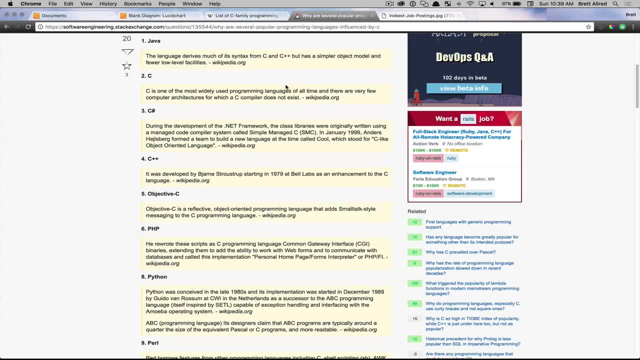 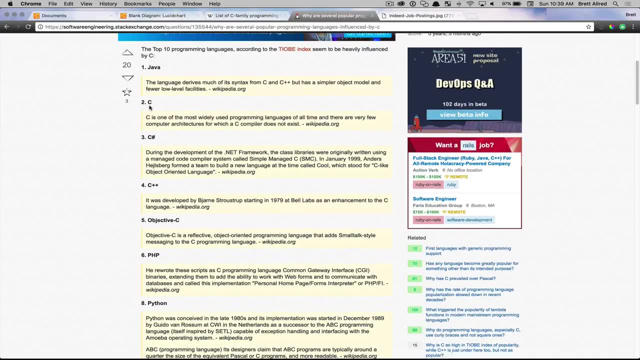 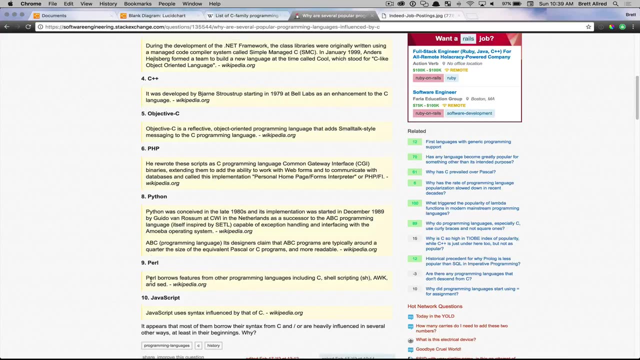 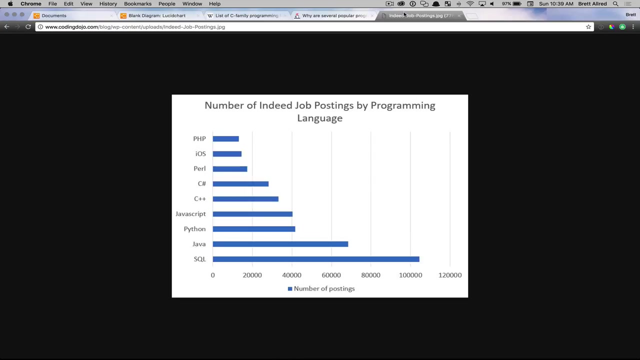 lots of them. so to make the list a little bit easier, I grabbed a top 10 programming languages that are heavily influenced by C, and here we have Java, we have C, obviously C sharp, C++, Objective C, PHP, Python, Perl, JavaScript. so those are probably the 10 most popular, and if you jump over to an, indeed job posting by: